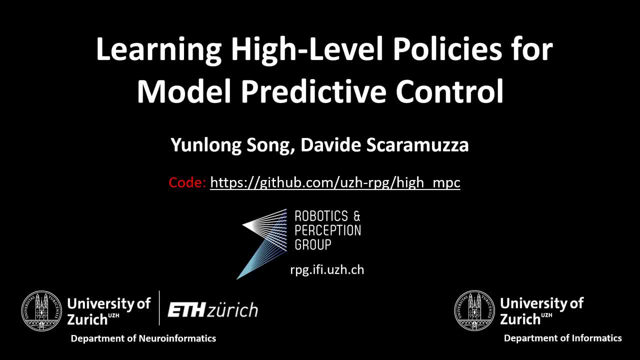 Hello, my name is Yunlong Song. I am a PhD student at the Robotics and Perception group led by Professor David Scalamuzza at the University of Zurich. We present our work on learning high-level policies for model predict control, which is a learning-based approach that combines policy search and MPC. 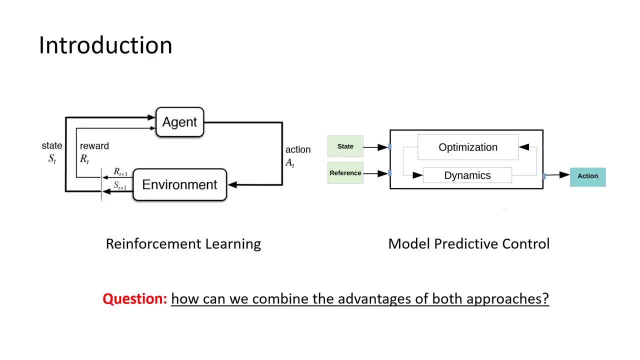 reinforcement learning, including deep reinforcement learning, is a useful tool for automating a variety of decision-making tasks. However, many reinforcement learning methods are extremely data inefficient and suffer from poor generalization. On the other hand, model predict control is a powerful approach for dealing with complex systems, with the capabilities of handling uncertainty and disturbance. 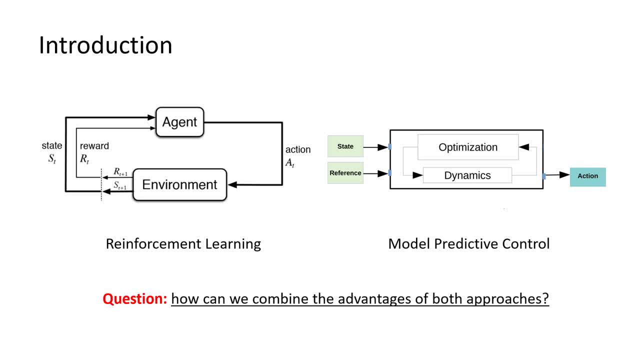 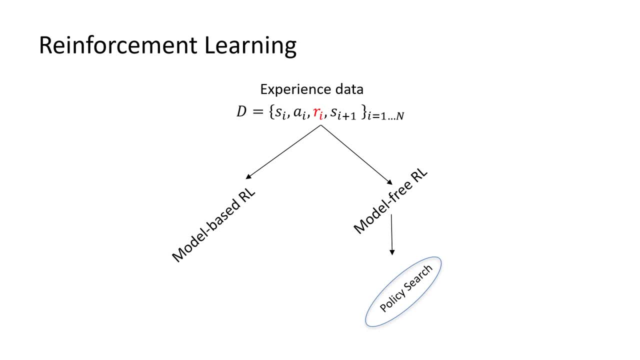 In this work we are trying to answer the question: how can we combine the advantages of both approaches? To do so, we make use of policy search, which is a model-free reinforcement learning approach that tries to optimize a policy directly from experienced data. 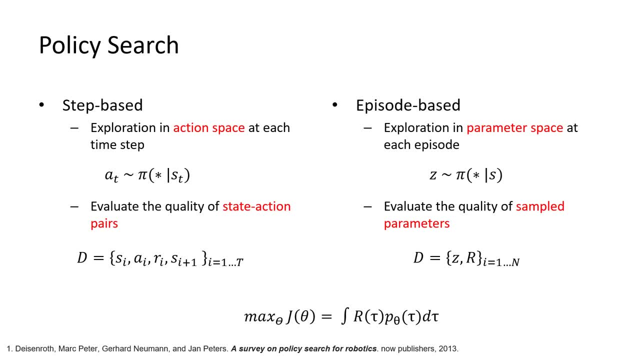 There are two kinds of policy search approaches: step-based and episode-based. Step-based policy search explores an action space at each stage, While episode-based policy search explores a parameter space at each episode. Both try to find a policy that maximizes the expected reward. 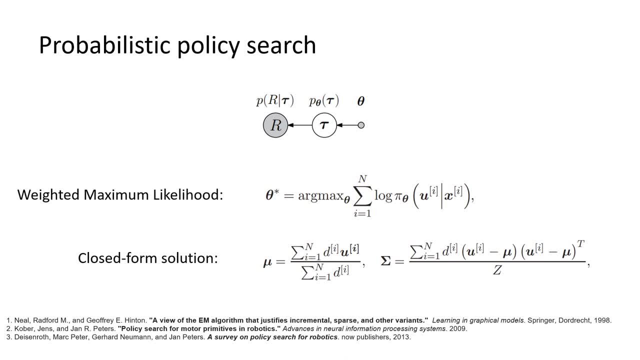 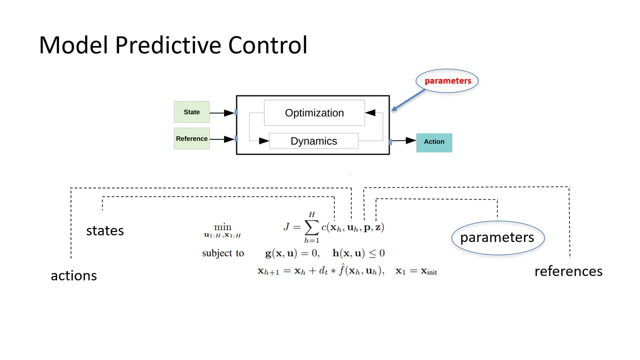 We use episode-based policy search. In particular, we use probabilistic policy search, in which the problem is formulated as a probabilistic inference problem and has an objective of the weighted maximum likelihood. This allows a close-on solution for the policy update Model predict control makes use of constraint optimization and the system dynamic for optimal control. 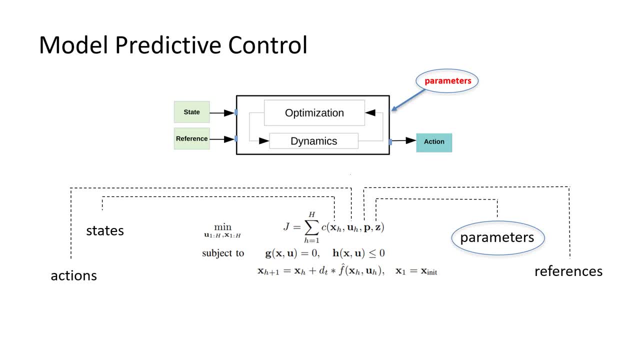 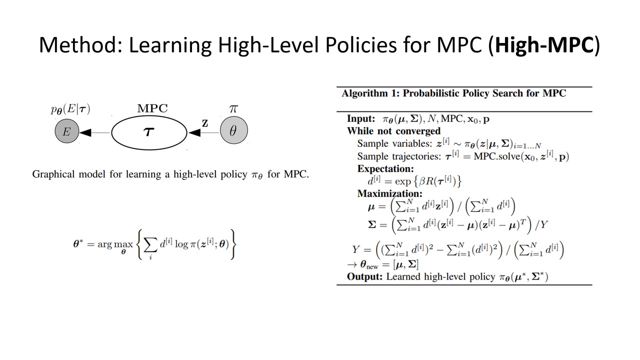 It takes states, references and some hyperparameters as inputs and outputs, the optimal control commands for the robot. Here the hyperparameters are normally designed by human experts. We formulate the search of hyperparameters in MPC as a policy search problem. We refer our method as learning high-level policies for MPC, in short, high MPC. 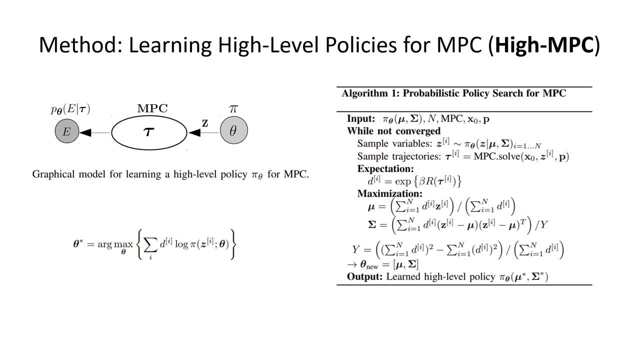 First we formulate the search of hyperparameters in MPC, which are also considered as high-level decision variables for MPC, as a probabilistic policy search problem. We model the parameters as Gaussian distribution. We make use of the multicolor expectation maximization approach for learning the policy parameters, since it allows a close-on solution for the policy update. 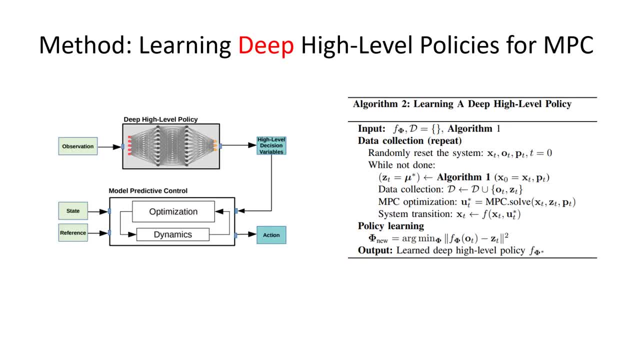 Second, we propose a self-supervised learning algorithm for learning a neural network high-level policy. by combining policy search with supervised learning Condition on a robot's observation in a changing environment, The trained policy is capable of adaptively selecting decision variables for MPC. 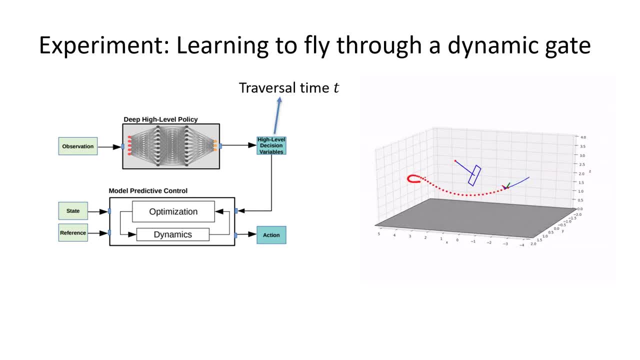 We evaluate the performance of our approach by solving a challenging robotic control problem where the task is to fly a quadrotor through a dynamic gate. In this case, the charge time is the high-level decision variable that has to be learned. On the left-hand side, we show the dynamic gate. 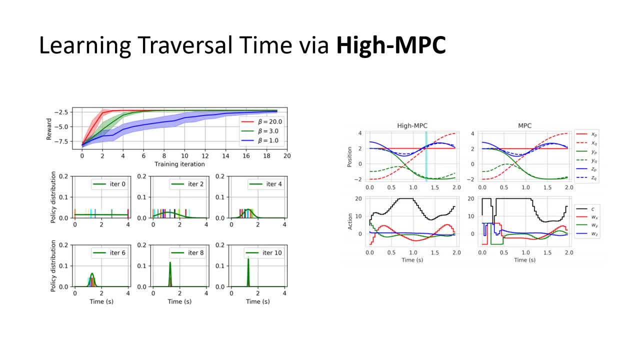 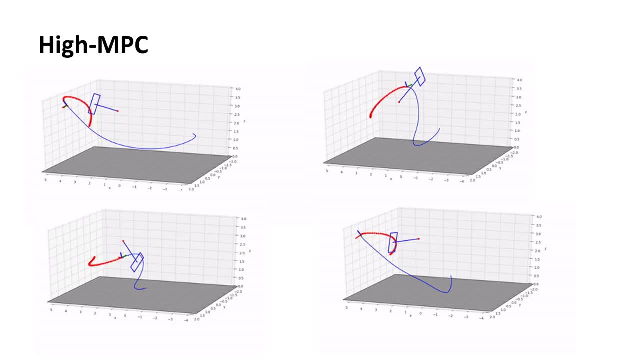 We demonstrate the robustness of our approach by randomly displacing the quadrotor inner space with random orientation. We demonstrate the robustness of our approach by randomly displacing the quadrotor inner space with random orientation. random orientation: our approach managed to fly through the gate even when the gate is moving very